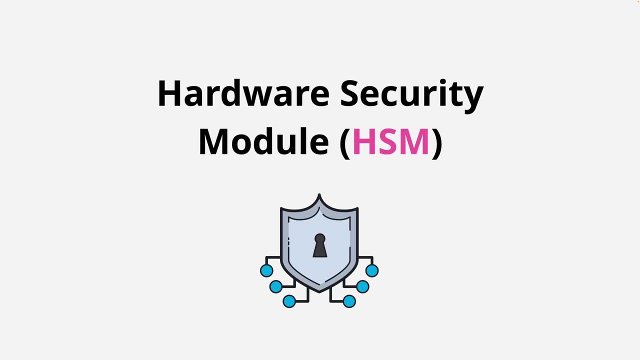 Welcome to this video where I want to talk at a high level about hardware security modules, known as HSMs. Now, these are a really important type of device to understand, both in general and especially if you currently work in or want to work in the security space, because so many other 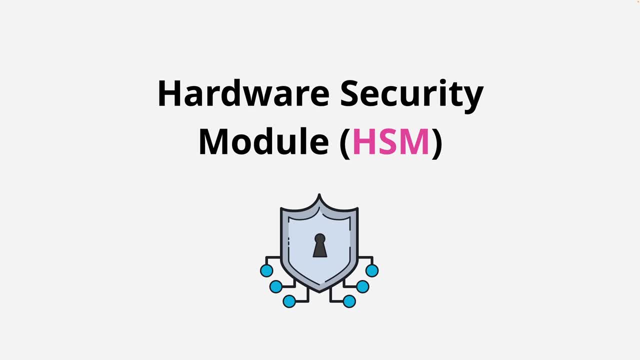 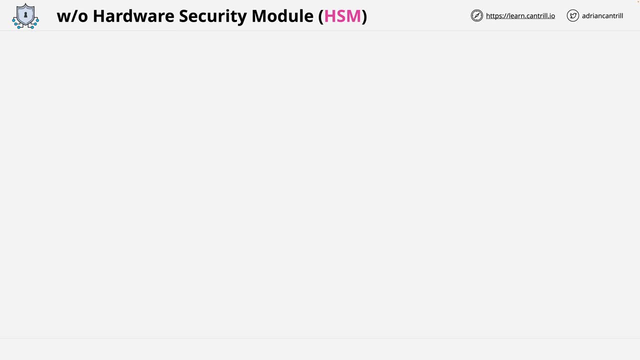 things rely on them to function. Now let's jump in and step through why we need them, what they are and how they work. Now let's start by looking at the world without hardware security modules, and we're going to do that with the example of a virtualized environment. and so we have a VM host. 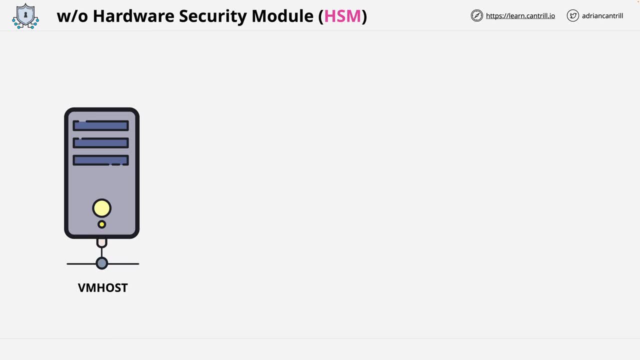 and this could be VMware, Zen or something within a cloud environment, It doesn't matter. for this example, This means that we have some physical CPUs, memory, as well as mechanical or solid state storage. Running on this is our hypervisor, a pair of operating systems, and to keep this, 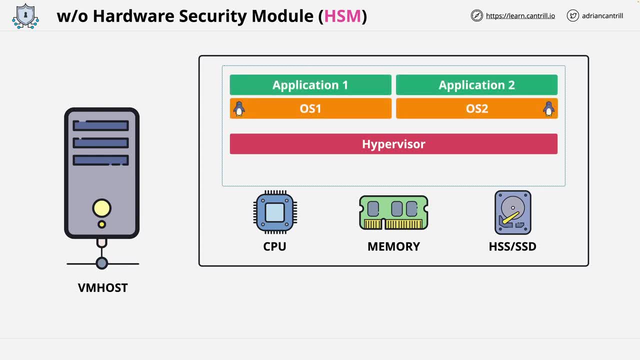 simple, a pair of applications. Now I want you to imagine that these applications, the operating systems and the hypervisor are all using encryption in some way. That might be encryption at rest or in transit, It might be public key infrastructure, or it might be simple SSL or TLS. Whatever the 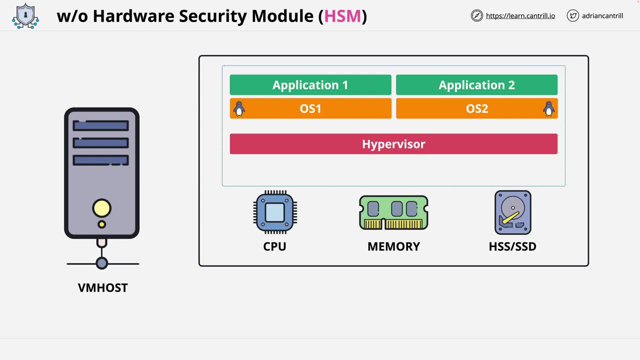 requirement. it means you're going to have keys stored in many places, Keys inside the applications controlled by the operating system or held by the hypervisor, And all of this means that keys will be handled by the CPU, held in memory and stored on storage And over time, if you care about disaster recovery, you're going to have 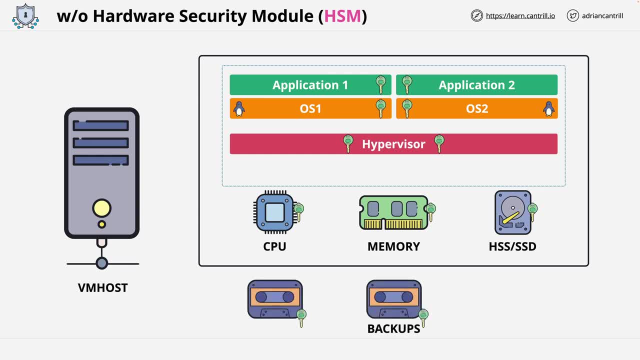 keys stored on various backups, some of which might go off-site for storage. Using encryption means using keys, and these keys will be stored or held in various places. You might think this is controllable, but over time they will leave your premises and because of this you're. 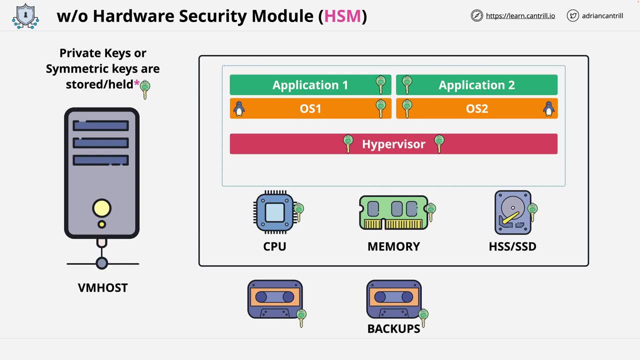 in direct control, meaning it becomes easier for these to fall into the wrong hands and become exploited. Now that's where HSMs add value. So let's take a look Now. this is a similar architecture, the same hypervisor, the same set of operating systems and applications and the same 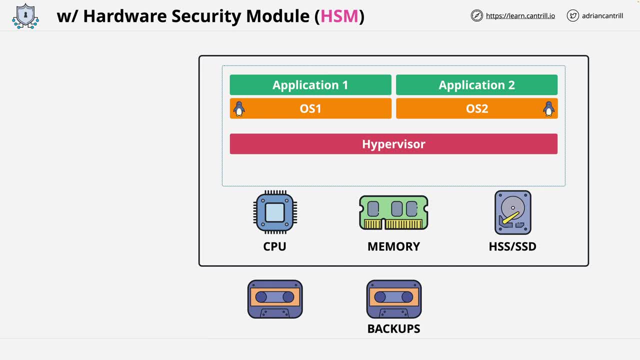 backup infrastructure. Only now we've chosen to utilize a HSM. A HSM or hardware security module, as the name suggests, is a separate device or cluster of devices. It's isolated from your main infrastructure And it's inside this device. 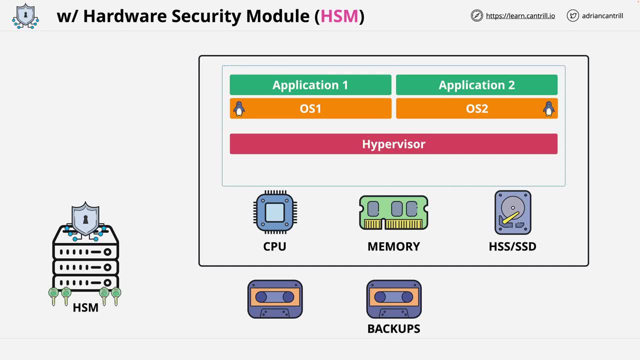 that your keys are stored. They never leave this device. They're managed by this device, often generated and deleted by this device. Anytime you want to perform cryptographic operations, you send those to the HSM together with the data. The HSM performs cryptographic. 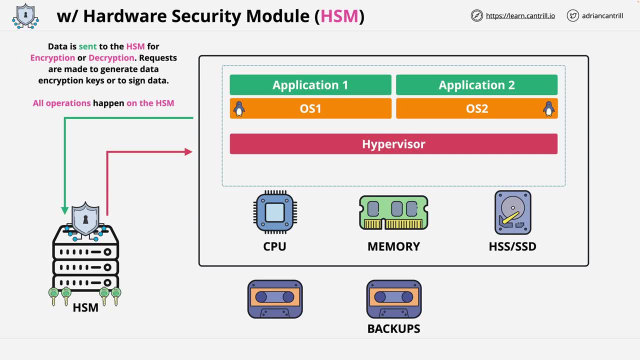 operations and sends the result back. It means you keep the same application and virtualization architecture, but instead of having to generate, manage, store and secure keys and risk those leaking with HSM, the keys are securely held on device. So that's HSMs at a high level. Let's finish by exploring the architecture in more detail. 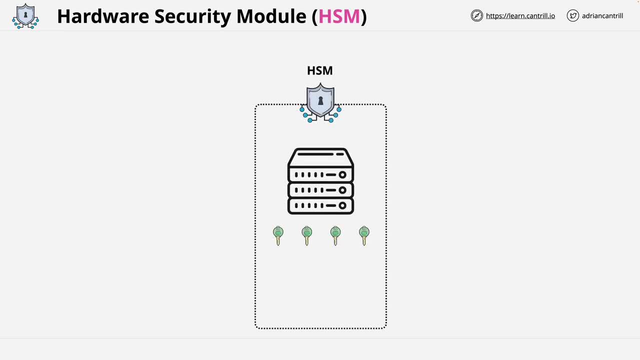 So now we have our HSM in the middle. Think of this as 100% separated from the rest of our infrastructure, accessible only in a highly defined way. Keys are created on the HSM, stored on the HSM, operations happen on the HSM and keys. 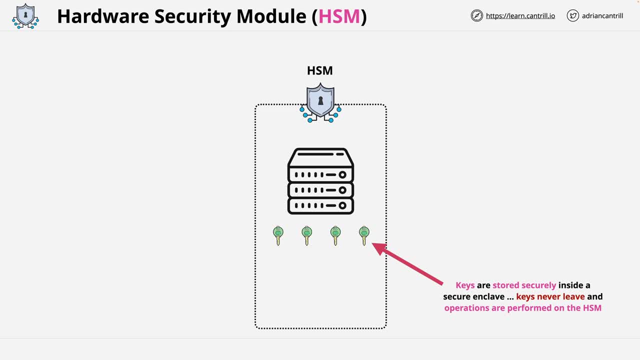 generally never leave the device. By utilizing HSM, you create a secure island within your infrastructure where all cryptographic operations are controlled. from Now, authentication takes place inside the device. This means you have an isolated security blast radius. Even if your corporate identity store was exploited, the identity store is 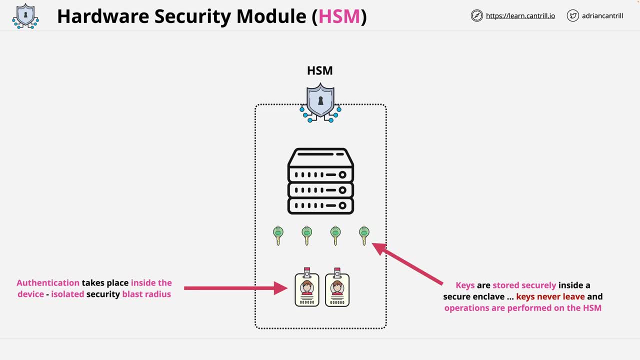 used within a HSM are internally defined and so can withstand this type of exploit. HSM's are tamper-proof and they're hardened against physical and logical attacks. The devices use secure enclaves internally, which makes it almost impossible to gain access to the internal key. 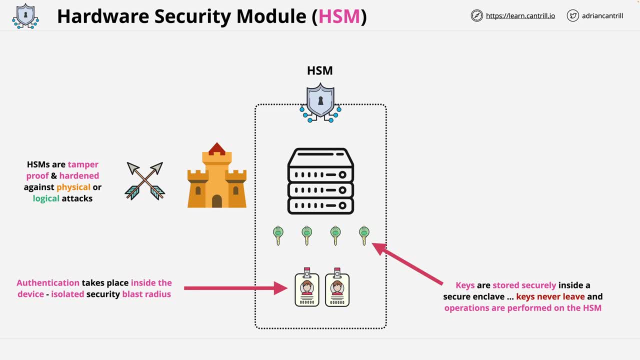 material through direct physical means. Many smartphones today come with a similar cut-down version of this. It stores your biometric information to keep it isolated from any badly behaving software on your smartphone. Access to cryptographic operations within the HSM is tightly controlled. You need access, but assuming you have those access permissions.